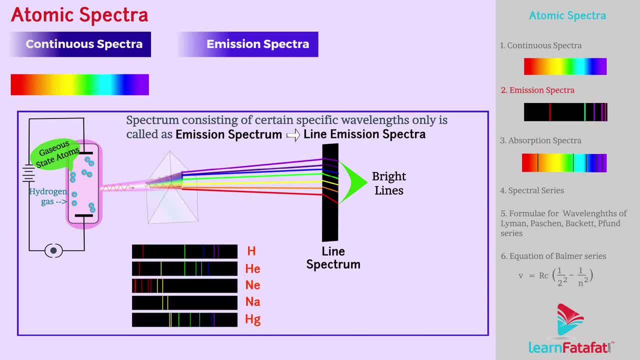 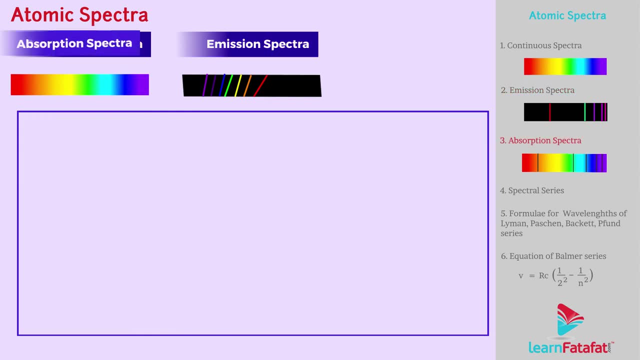 Each element have unique Line Emission Spectrum. By comparing the Line Emission Spectrum emission pattern of unknown element to that of known standard pattern of elements, it is possible to identify the element Absorption Spectra If white light is passed through the gas. 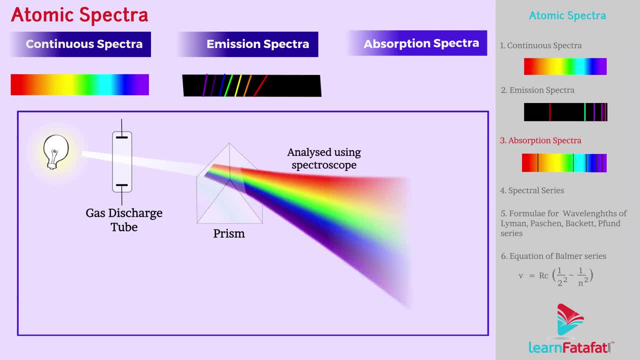 the transmitted light is analyzed using spectroscope, then it gives some dark lines on bright background. Such spectrum is called the absorption spectrum of the material of the gas. These dark lines correspond precisely to those wavelengths which were found in the emission line spectrum of the gas. 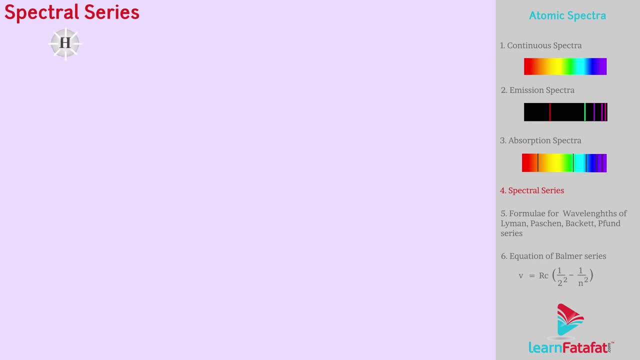 Spectral Series. Dear students, Hydrogen is the simplest atom and therefore has the simplest spectrum. When the spectrum of hydrogen was observed, there was no regularity observed in spectral lines. However, the spacing between lines go on decreasing after few set of lines. 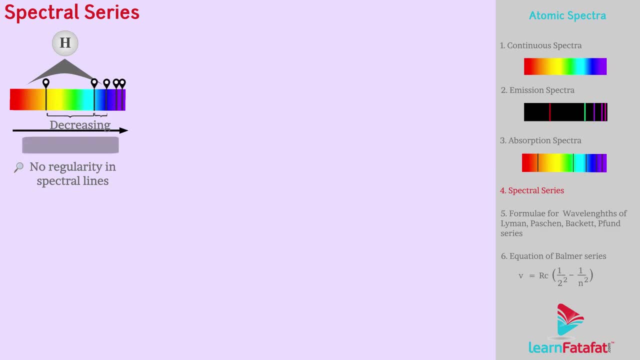 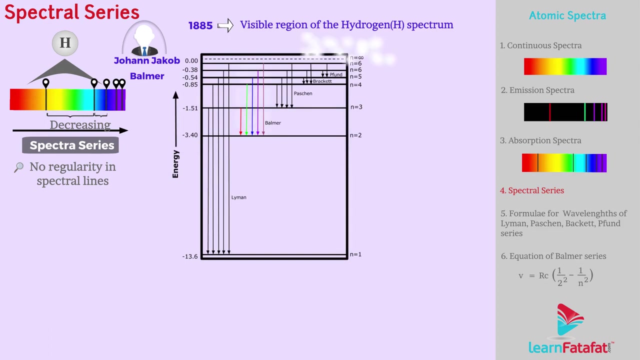 Each of these, set in emission pattern, is called Spectral Series. Johann Jacob Barmer observed the first such series in 1885 in the visible region of the hydrogen spectrum Spectral Series. This series is called Baamir series. The line with the longest wavelength, 656.3 nanometer, in the red is called H-alpha. 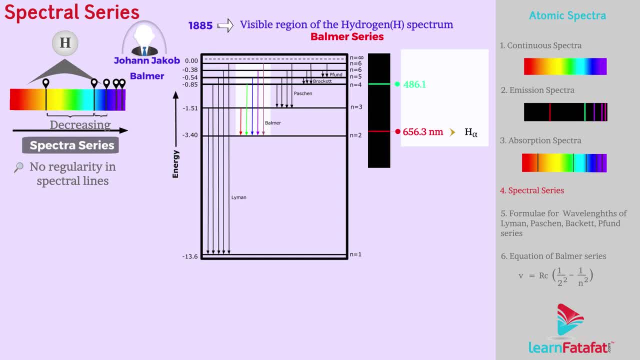 The next line with wavelength 486.1 nanometer in the blue-green is called H-beta. The third line, 434.1 nanometer in the violet, is called H-gamma, And so on up to H-infinity. Baamir derived a simple empirical formula to find the observed wavelength. 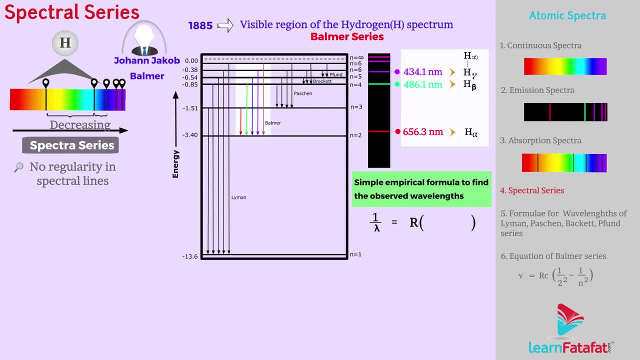 It is given as 1 by lambda equals to r, into bracket 1 by 2 square minus 1 by n square. This equation is also called Baamir formula, Where lambda is the wavelength, r is a constant called the Rydberg constant.